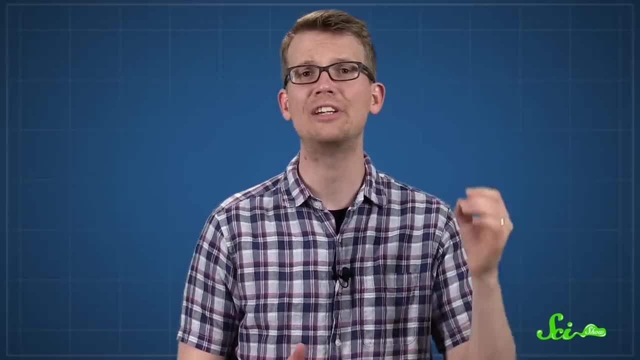 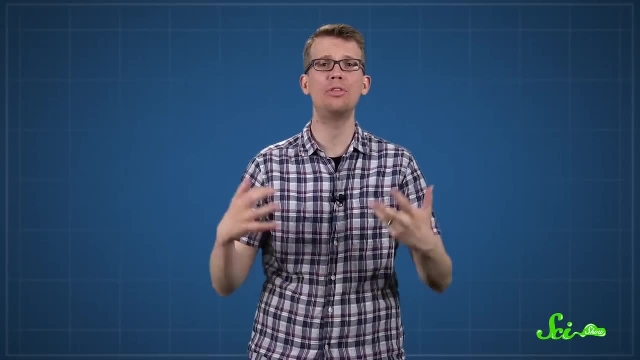 ancient life of all kinds, mostly, but not always, by investigating fossils, the mineralized remains of living things. It kinda makes sense that the two fields are often confused for each other, because they both use science to understand history and they both involve a lot of digging. 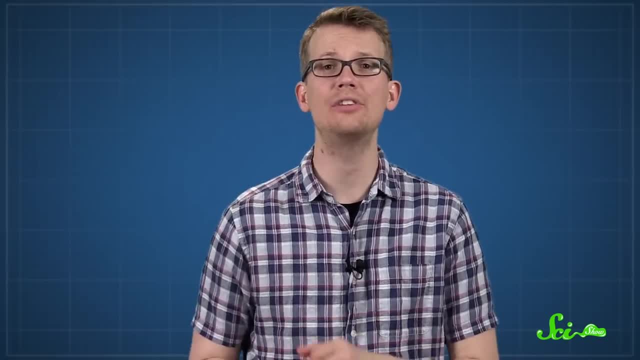 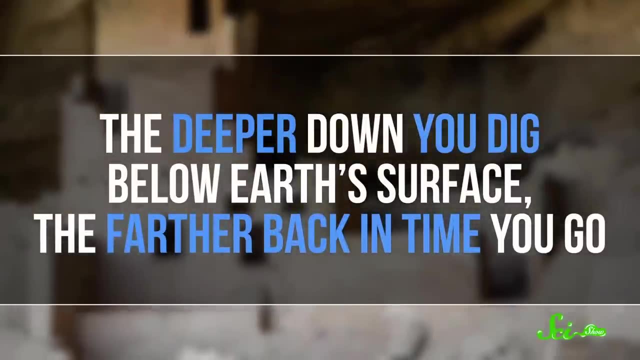 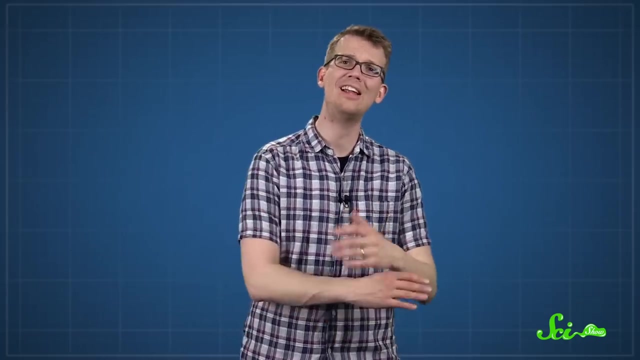 In fact, the main thing that archaeology and paleontology have in common is the basic understanding that the deeper down you dig below Earth's surface, the farther back in time you go. The surface of the Earth is always reworking itself, after all, whether it's because of plants dying and turning into topsoil, or volcanic eruptions covering everything in ash, or floods laying down new layers of sediment. 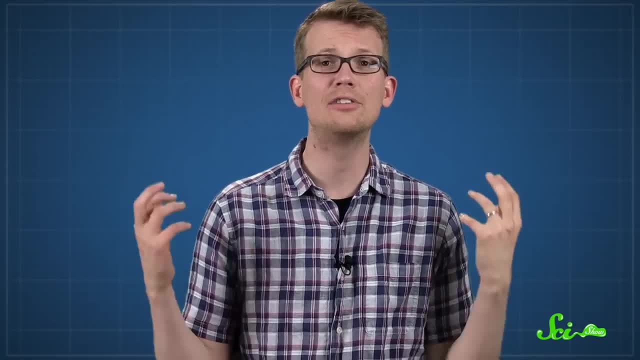 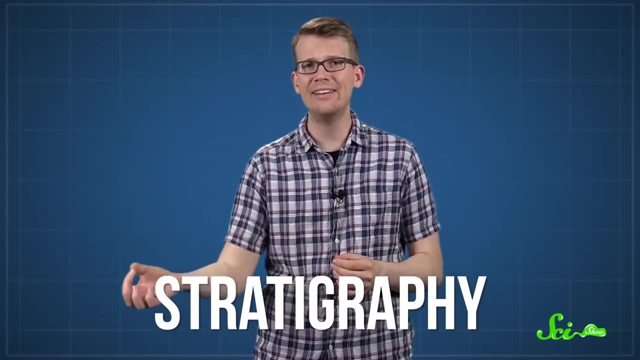 That's why both archaeologists and paleontologists are trained in the science of reading these layers, a branch of geology called stratigraphy. But that's about where the similarities end, because archaeologists and paleontologists explore the strata of Earth at different depths, looking for different things. You might not have to dig too far to find, like stone, spear points from a few thousand years ago. but to reach back further into the past and find a fossil of a pteranodon you gotta get into older layers of Earth. 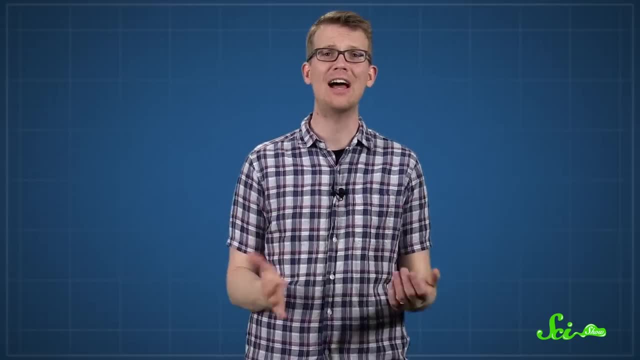 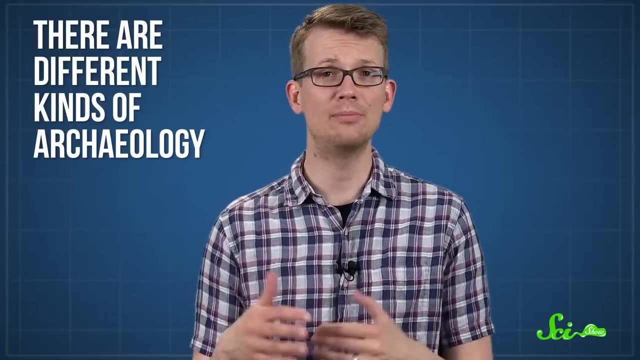 So archaeologists study human history, but humans have been around a long time and we've left a lot of history lying around, so it makes sense that there are different kinds of archaeology. Since most of our history hasn't been written down, a lot of archaeologists study prehistory. 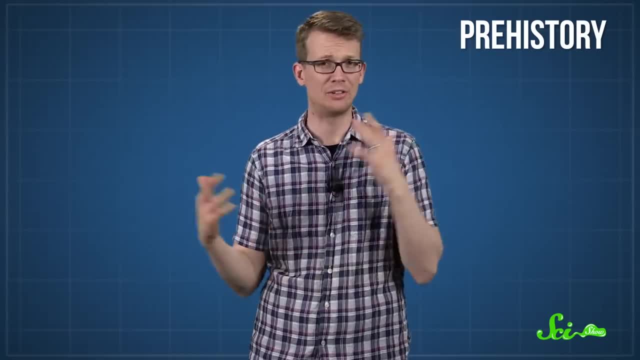 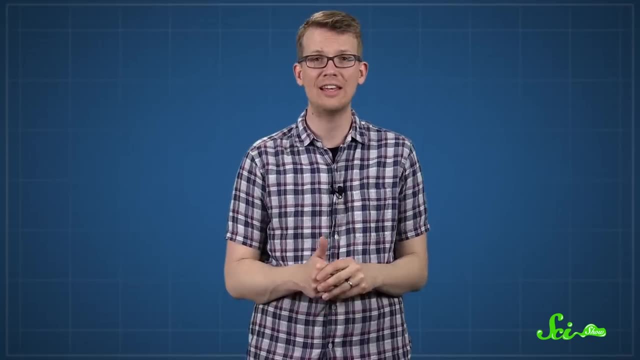 Now, prehistory doesn't mean before there was history- obviously there's always been history- But simply a time before history. Historical events were actually documented either in writing or in oral traditions. that can help us understand what we find in the ground. 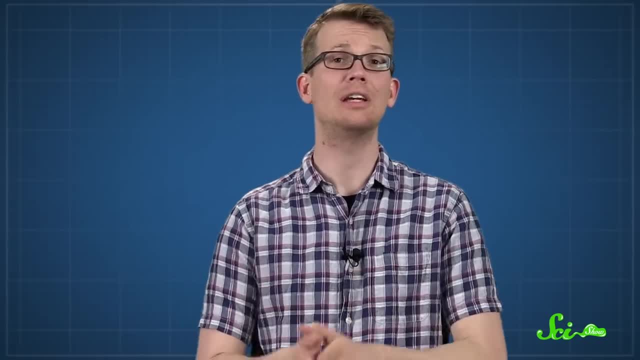 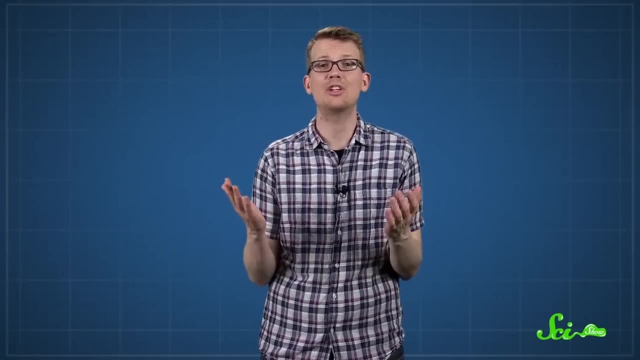 So the investigation of cultures that thrived before they fixed their history into words is prehistoric archaeology. The Stone Age dwellers of the Levant, the hunter-gatherers of America, even the cultures that created Stonehenge and the great houses of Chaco Canyon all fit into this category. 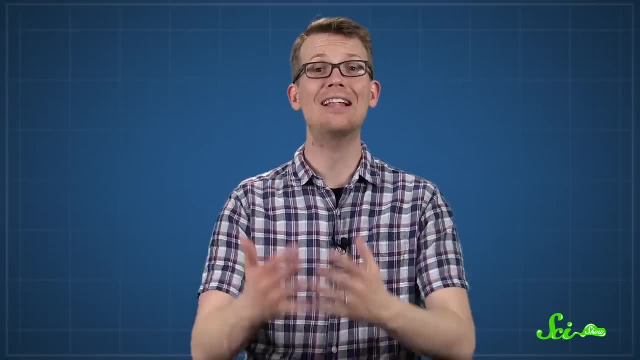 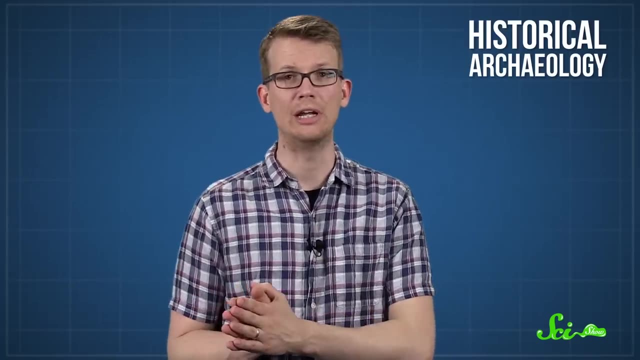 But even after historical records started to become a thing, there were still lots of gaps for us to fill in. So historical archaeology is dedicated to exploring the history of the world, Exploring the lives of people who lived during recorded history. Classical archaeology, for example, focuses on ancient Western cultures like those of Greece and Rome. 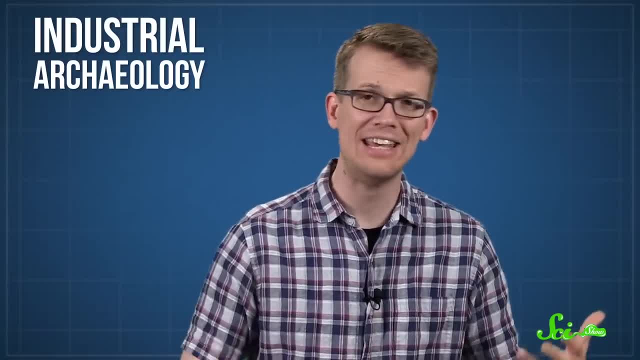 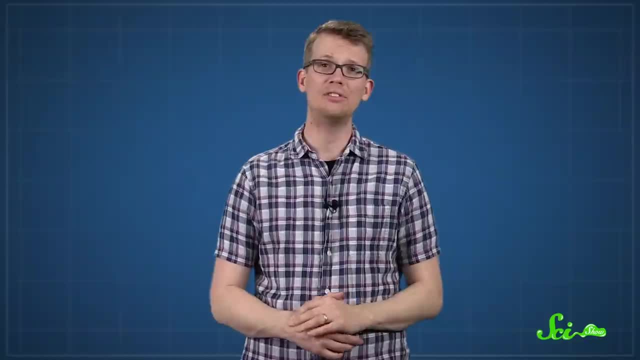 Industrial archaeology explores old ways of engineering, mining and manufacturing. There's even a whole subfield of maritime archaeology which just investigates shipwrecks. None of these fields, you'll notice, involve raiding tombs or snatching golden idols from booby-trapped chambers, or punching Nazis.